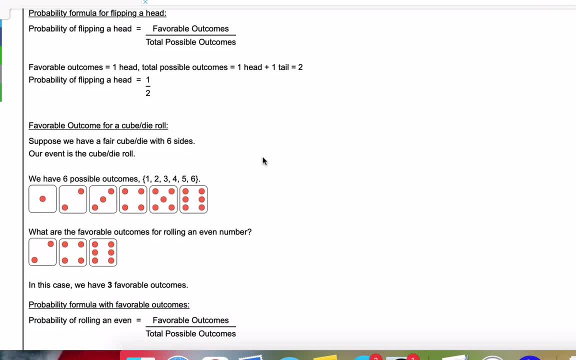 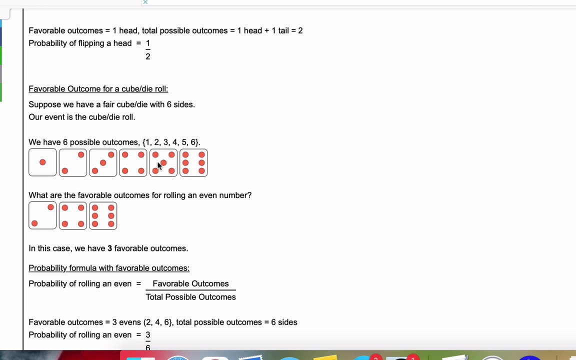 using a cube or a die roll. We're going to take one six-sided cube or die. It's fair, meaning equally weighted on all sides. Our event in this case is the cube or the die roll. We have six possible outcomes or total outcomes. We can roll a one, two, three, four, five or six. They're all. 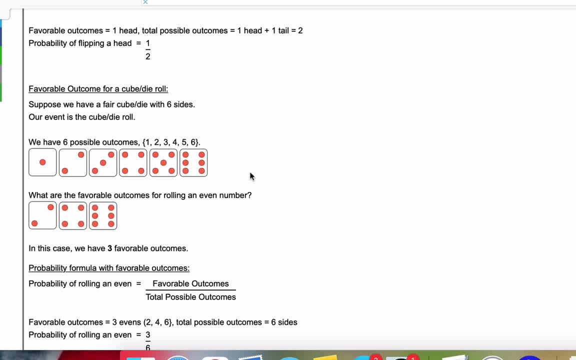 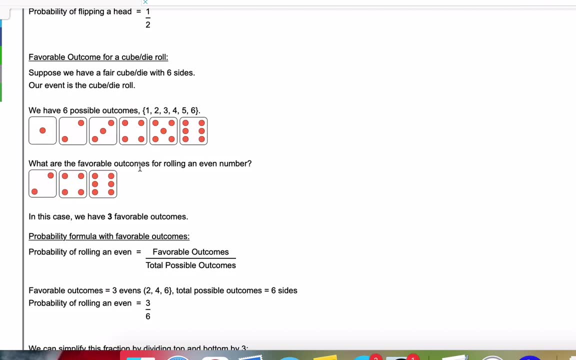 equally weighted. Suppose we want to ask what are the favorable outcomes for rolling an even number? Well, one through six, we have three even numbers. We've got two, four and six. In this case we have three favorable outcomes. Now how does it all tie in and wrap up into probability? We're going to 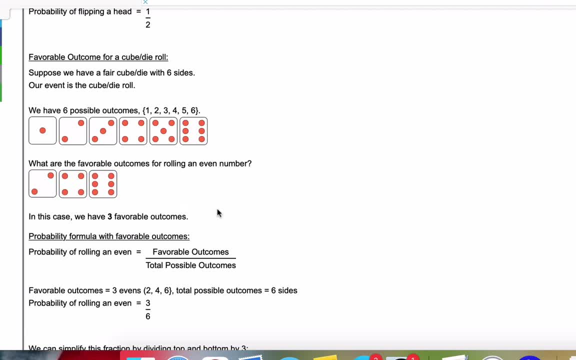 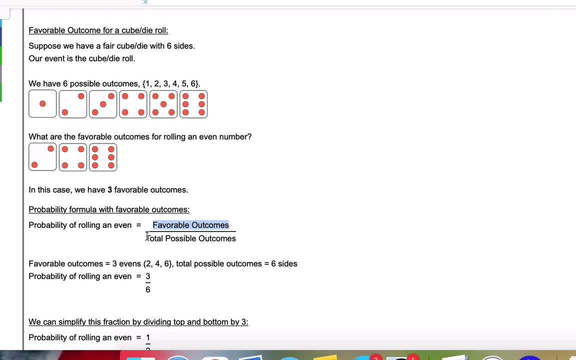 use the same formula we use for the coin flip as for the cube or die roll. So, once again, the probability of rolling an even is the number of favorable outcomes divided by the total possible outcomes. In this case, the favorable outcomes are three, since we have three even faces, two, four. 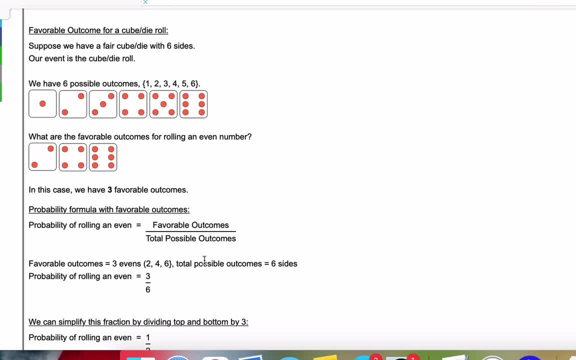 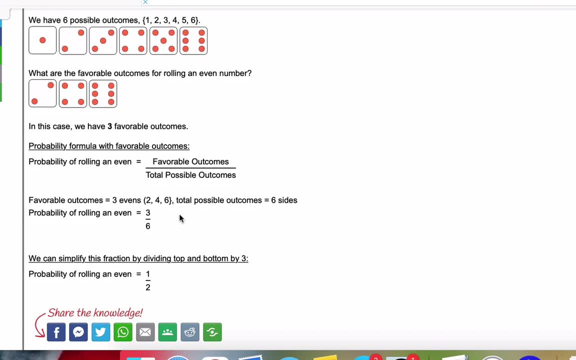 and six, And the total possible outcomes in this experiment is six for all six sides up here. We plug these numbers in and we get the probability of rolling an even is three-sixths. Now if you use our greatest common factor calculator. 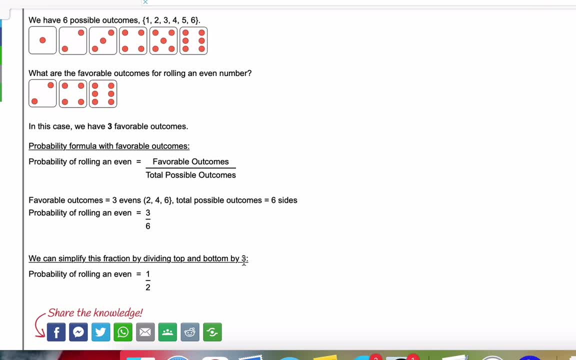 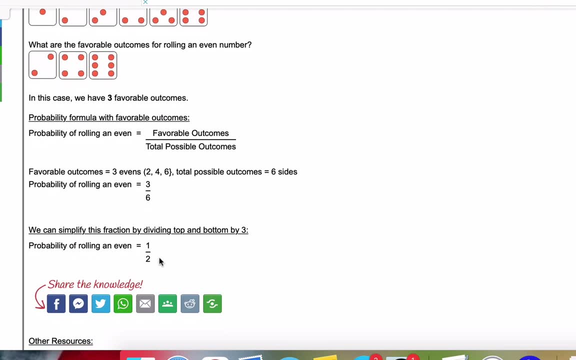 you'll see that the greatest common factor of three and six is three. We divide each of these two by three and we get the simplified probability of rolling an even is one-half. So that is favorable outcomes in a nutshell, And the question I get most is: what does it? 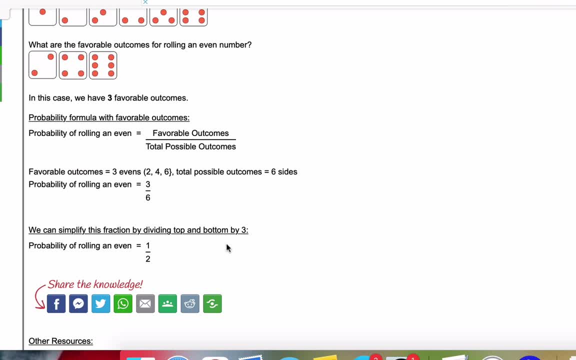 matter for favorable outcomes. All you care about for favorable outcomes is: how many possible ways can I get what I'm looking for? And I may be looking for flipping ahead, but I'm not looking for flipping ahead, Flipping a tail, rolling a four. I may be looking at marbles in a jar which we'll cover in another. 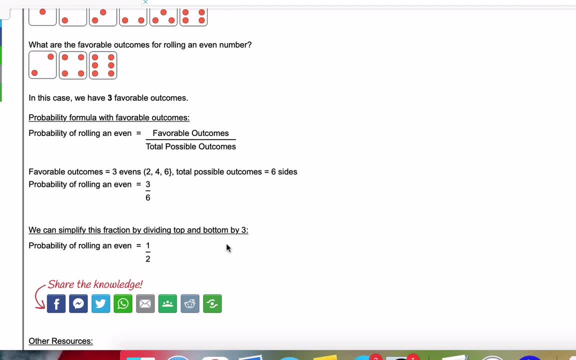 video. Probability in these cases is: how many ways am I looking for versus how many total ways can something happen? So that is it, my friends. I want to thank you for watching this video and I will see you in the next video. Subtitles by the Amaraorg community.